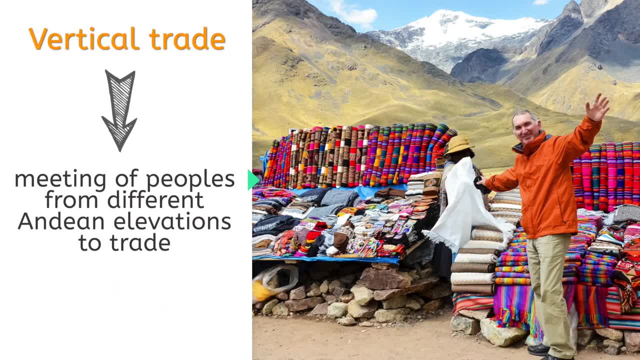 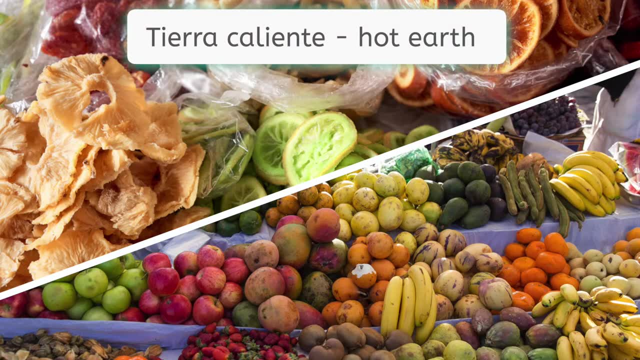 differing elevations in Andean market towns to barter their crops and handmade goods. Bananas, sugar and other fruits grown in the tierra caliente, or hot earth, may be swapped for potatoes and cabbages from tierra fría, or the cold earth. 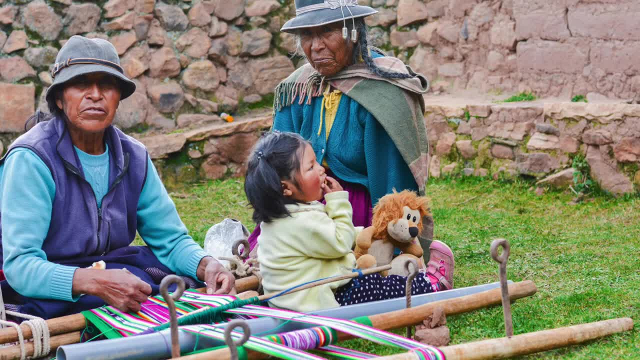 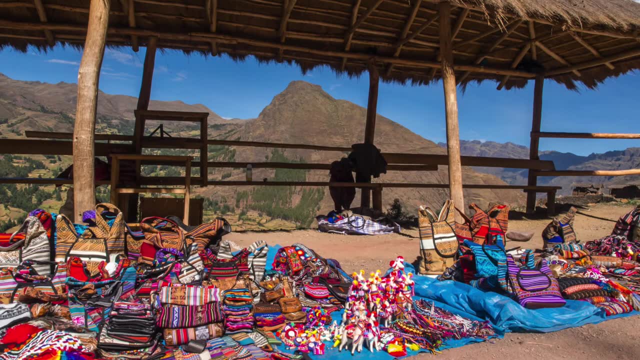 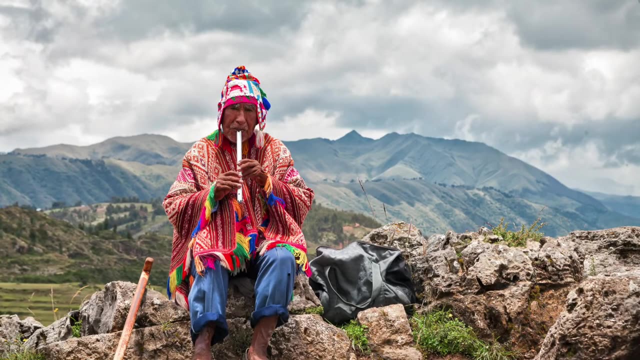 The fact that such a tradition has endured for centuries isn't surprising when you learn that the Andean nations of Bolivia, Ecuador and Peru have all been very successful. While Spanish is the official language of each, it's mixed with multiple indigenous languages, such as Quechua, common in all three nations. 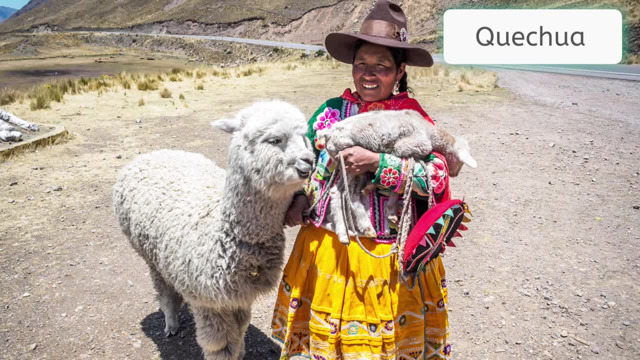 The Quechua, who predate the Incan civilization, live even today in the Andes at altitudes as high as 17,000 feet or more than three miles above sea level. Because of the altitude, the air is thin and the Quechua have developed unusual physical 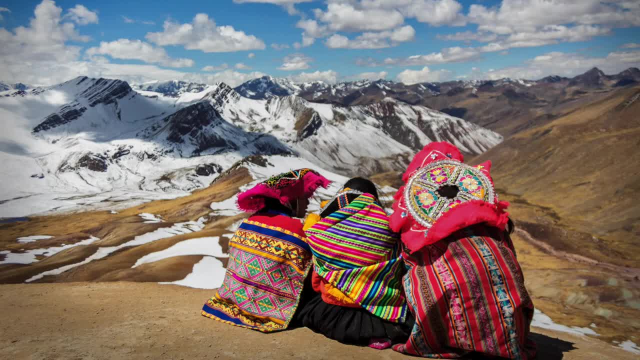 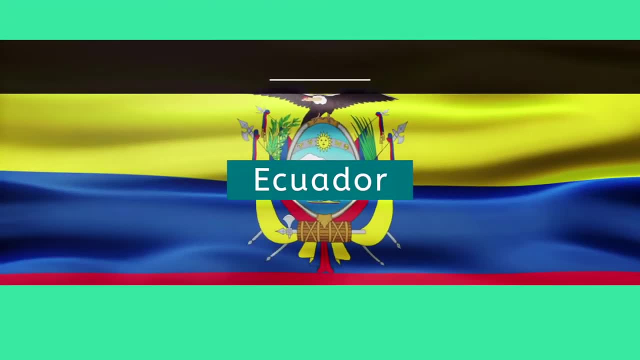 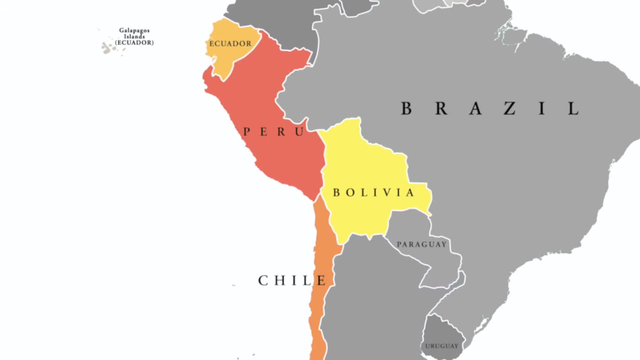 characteristics such as larger homes, high sea levels and more than one-third of the larger hearts and lungs similar to their mountainous peers on the other side of the world, the Sherpa people of Nepal, Ecuador. Four South American nations are part of the Andean region: Ecuador, Peru, Bolivia and Chile. 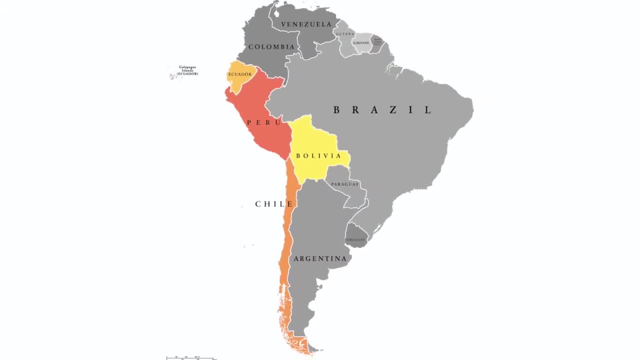 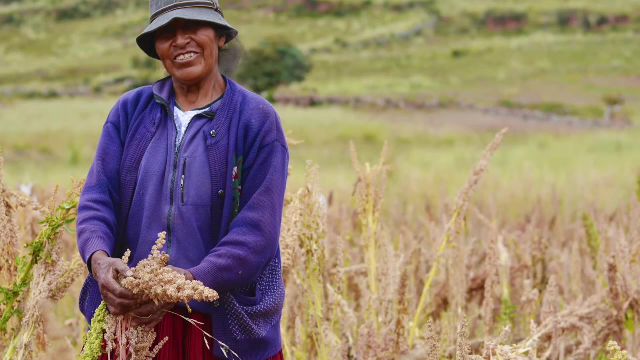 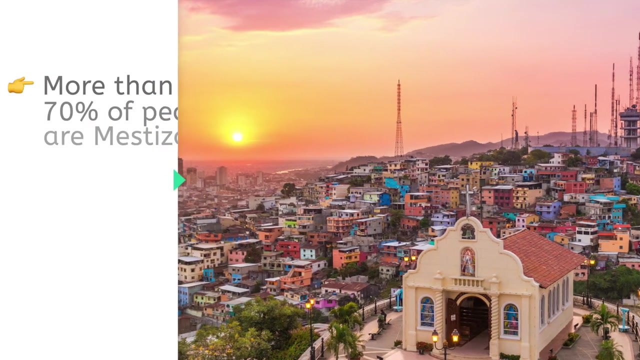 The Quechua people are found in all four and make up about one-fourth of Ecuador's 17.7 million people as of 2021.. They reside in the Andes and practice subsistence farming for survival, much like they did centuries ago, But more than 70% of the population of Ecuador is of at least 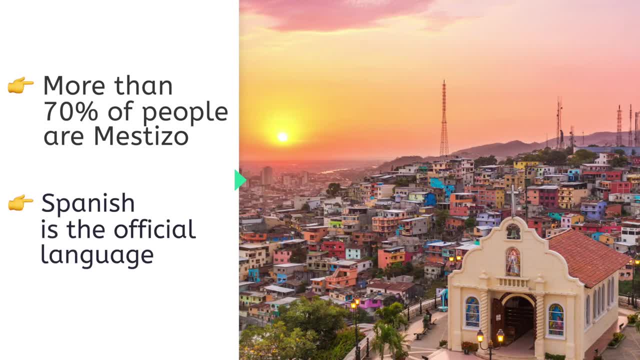 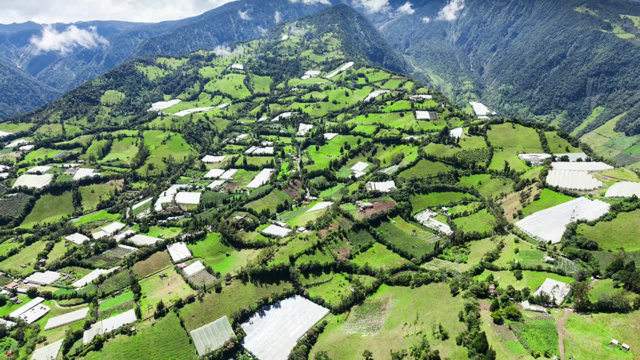 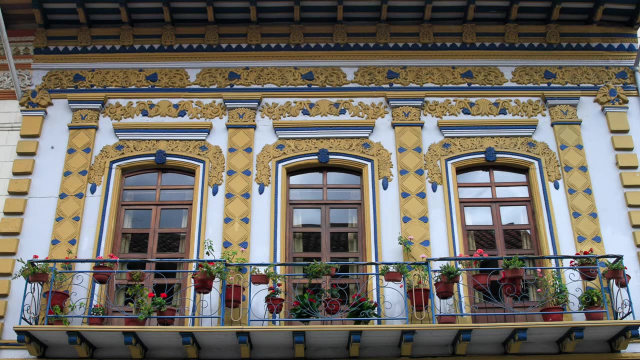 partial European descent, Spanish-speaking mestizos who practice Catholicism and work mostly in factories and tenant farms. The people are distributed fairly evenly between the highlands and the coastal lowlands. The affluent in Ecuador are those of direct Spanish heritage, which make up no more than 10% of the nation's population. 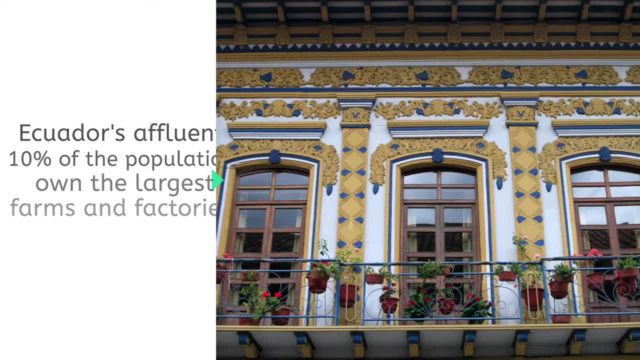 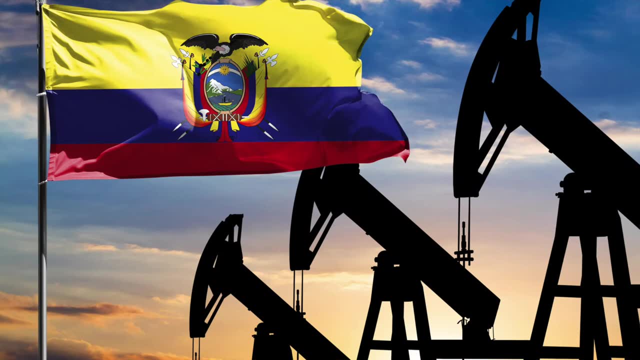 and who own the largest farms and factories and, predictably, have the most political influence. Petroleum was discovered in the selva in the 1960s and quickly became a vital export for Ecuador. However, fluctuating oil prices and government mismanagement led to economic instability. 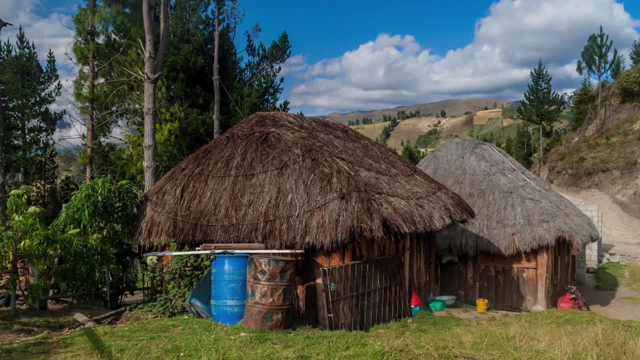 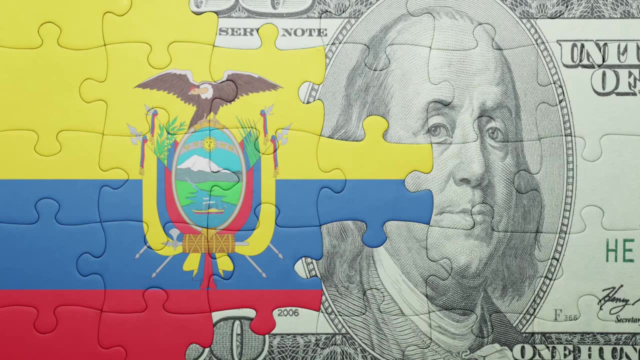 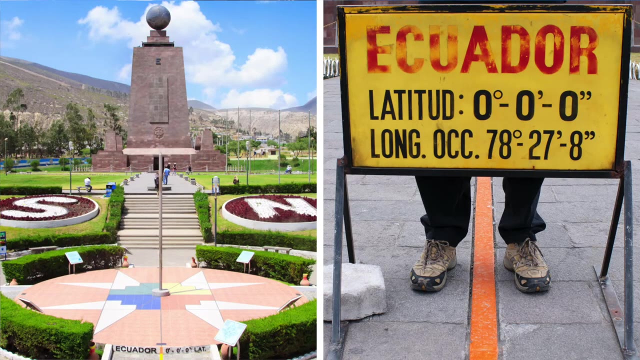 By 2000,. roughly 40% of the population lived in poverty. Adoption of the US dollar over the traditional Ecuadorian Sucre and investment in education and healthcare since then have stabilized the now improving economy. Two geographic notes about Ecuador. First, as you might have guessed, the nation gets. 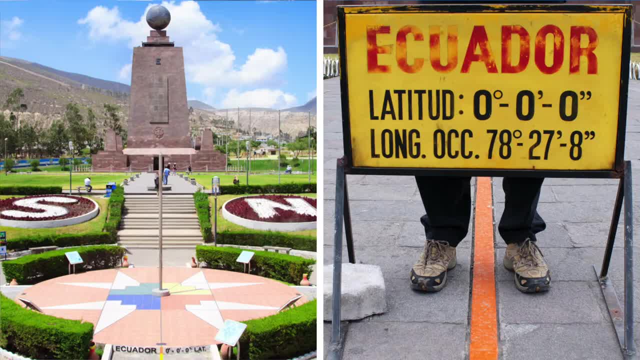 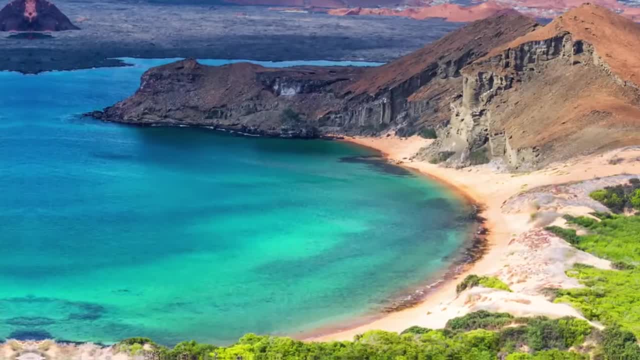 its name from the equator, which passes through the heart of the nation. Second, the Galapagos Islands lie 563 miles off the Ecuadorian coast. The islands, also called las encantadas or the enchiladas, are known by the Italian quantity They also have. 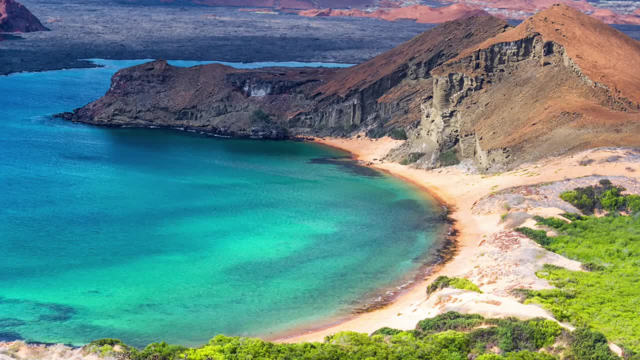 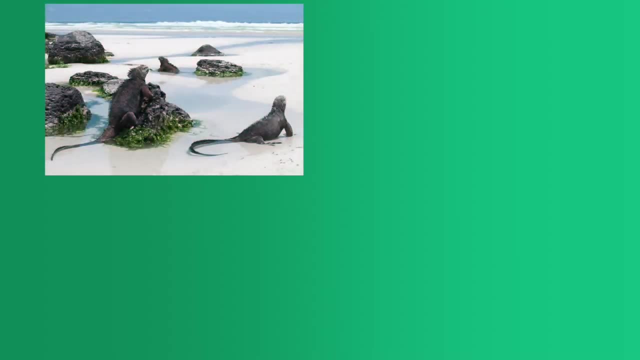 a very unique or singular subtype of food. in them, For example, the Basque cheese is a good. the Enchanted Isles are an Ecuadorian national park and protected environmental area, and are also home to noteworthy species such as marine iguanas, sea cucumbers, blue-footed boobies. 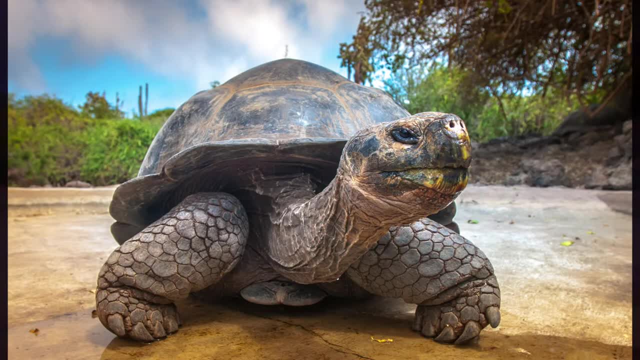 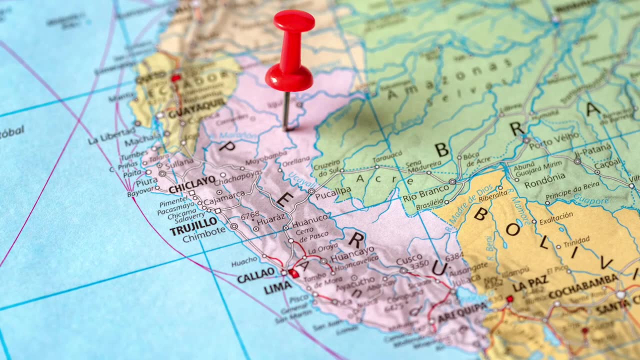 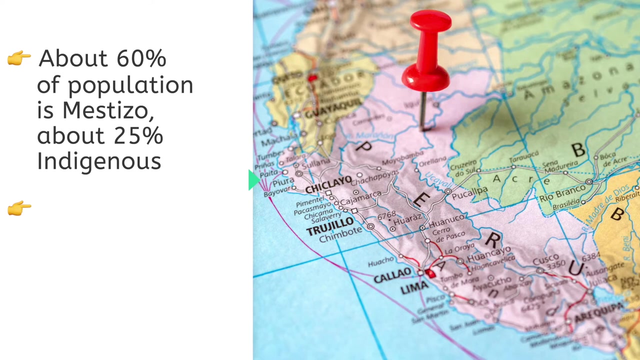 sea lions and the famous Galapagos tortoise. Peru: The demographics of Peru are similar to those in Ecuador. About 60% of the population is Spanish-speaking mestizos, while about a fourth of the people are indigenous, most of whom are Quechua, a language which is also an official language, Similar to much of. 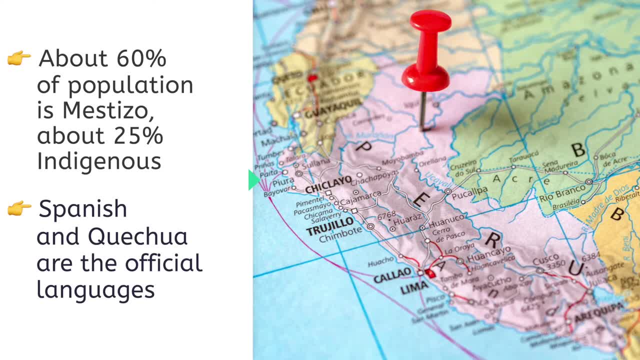 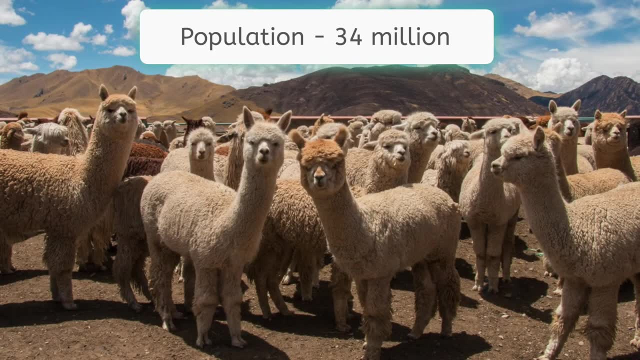 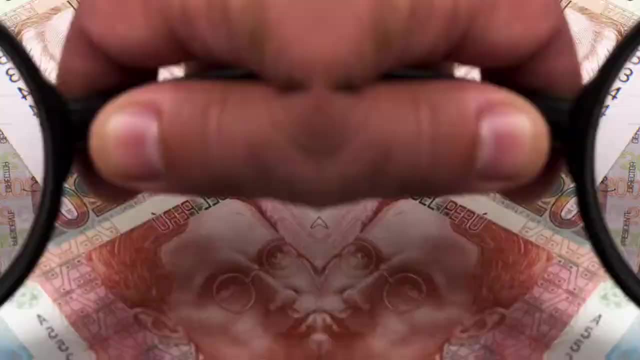 South America. more than 75% of the population is Roman Catholic. Many of the 34 million Peruvians are subsistence farmers or llama and alpaca herders. Others live in cities on the coastal plains and work in factories, mines or on large plantations. Economic conditions in Peru have 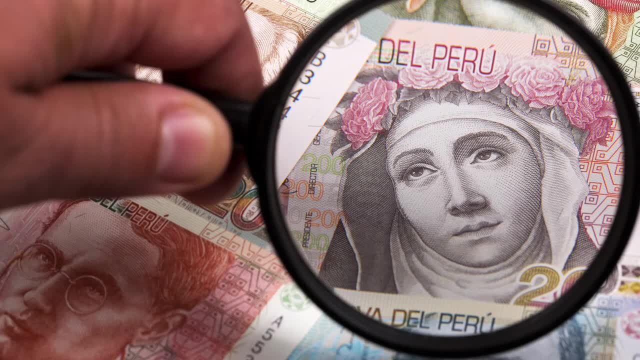 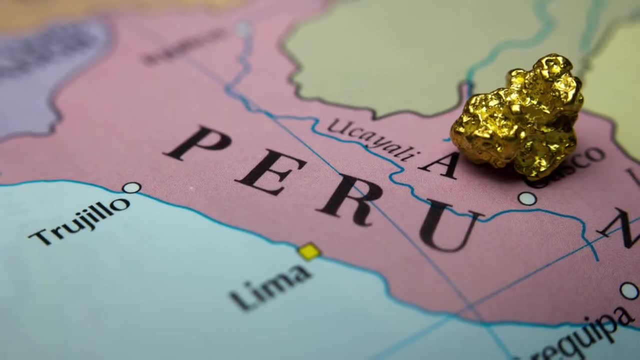 improved, but the population has not been as good as in the past. Since the early 2000s, Peru has had one of the fastest-growing economies in the world. Mined exports such as copper, gold and petroleum bring money to the nation. 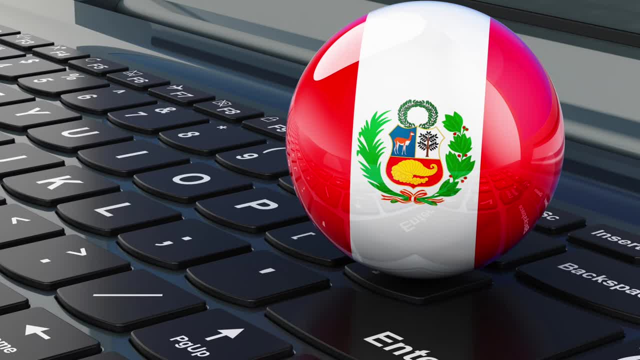 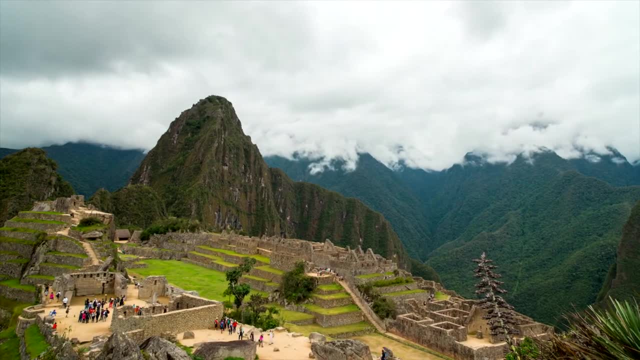 and an expanding base of tertiary services has also added to the nation's GDP. Still, Peru is best known for being the heart of the vast Inca Empire, which fell to the Spanish in the early 1500s. Tourists today still flock to the Andes to walk. 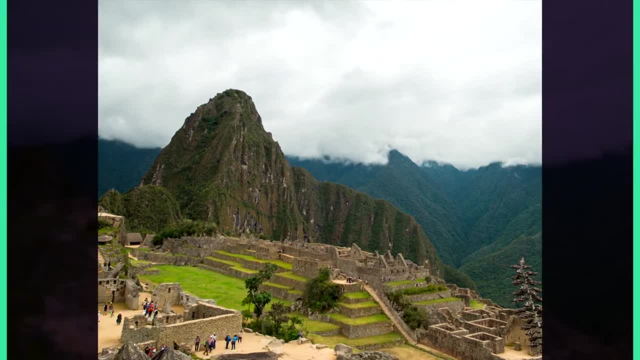 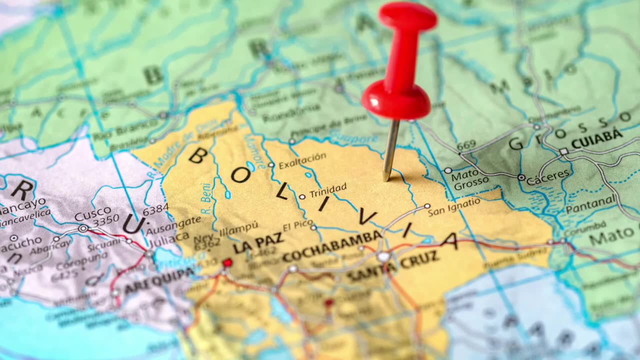 the ruins of Machu Picchu and relive a bit of history. Bolivia, One of only two South American nations that doesn't border either the Pacific or the Atlantic Oceans. Bolivia, as you probably recall, is named for El Libertador Simón Bolívar. 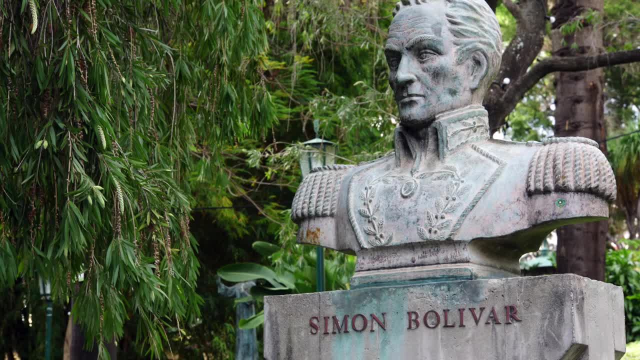 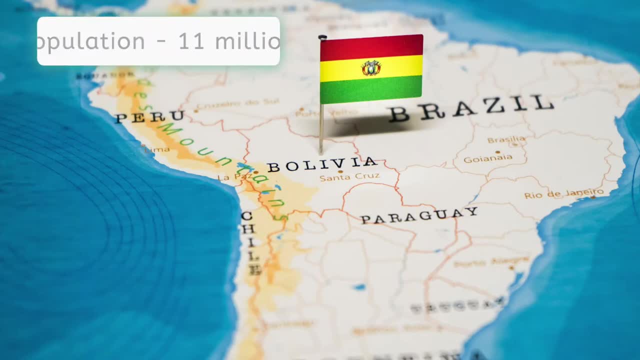 who led and inspired revolution in many South American countries. Although the Bolivian government did not include Mestizo as a choice in its 2012 census, most of the 11 million citizens are Mestizo, But with the indigenous component higher than the European. 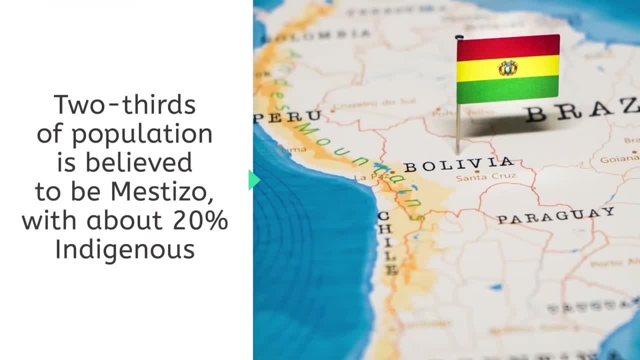 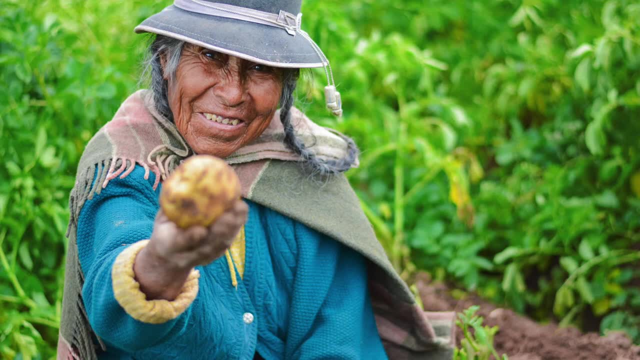 A 2018 estimate of the Bolivian population identified some two-thirds as Mestizo, with about 20% indigenous. Most Bolivians are subsistence farmers living in the highlands. Crops vary based on climate, which changes based on the altitude. 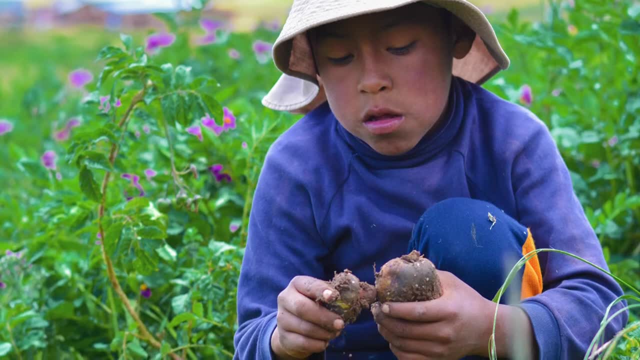 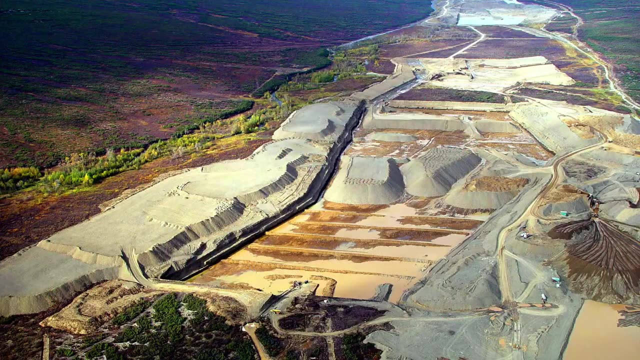 The climate ranges from cold and semi-arid to humid and tropical Farming, while a way of life for many is not as vital to the nation's economy. Natural gas, Gold and zinc drive Bolivian business. Still, Bolivia, as of 2021, was the second poorest nation in South America. 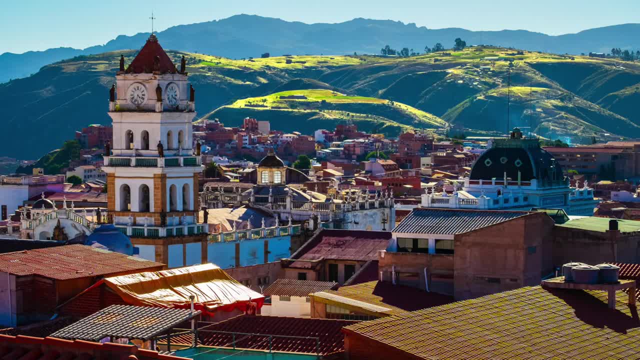 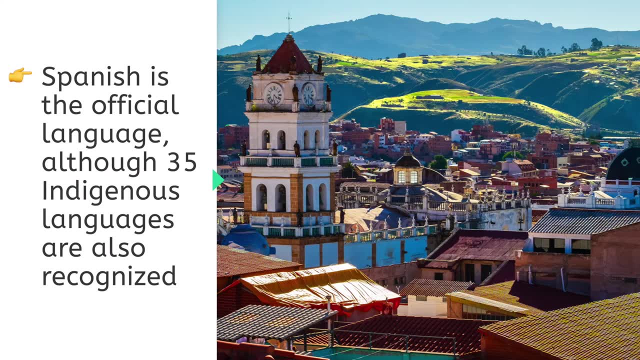 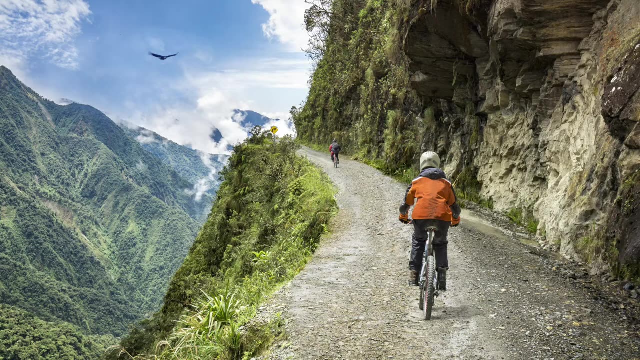 Like most of South America, Bolivia is predominantly Catholic and speaks Spanish, although the nation has 35 other official languages, all indigenous, the largest of which is Quechua. Other than Bolivia's status as one of the only two landlocked South American nations, Paraguay being the other- 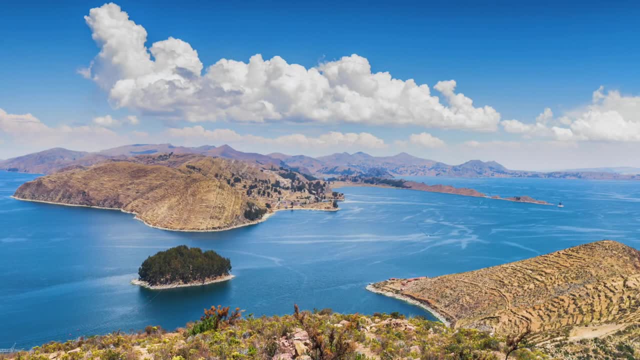 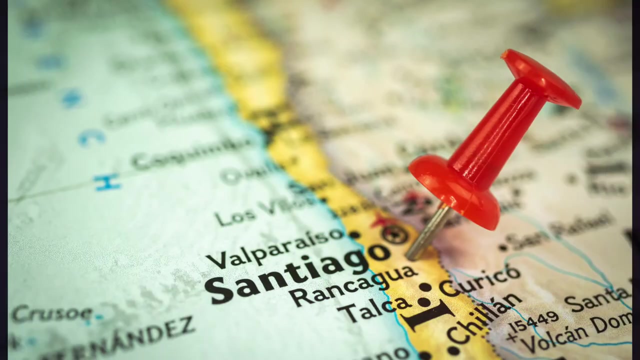 another geographical mention goes to Lake Titicaca. As the highest navigable lake in the world, Titicaca sits in the Andes, on the border between Bolivia and Peru. Chile- Appropriately, Chile in the indigenous Mapuche language means end of the land. 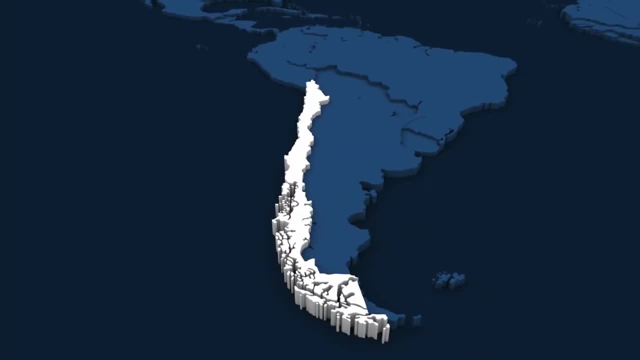 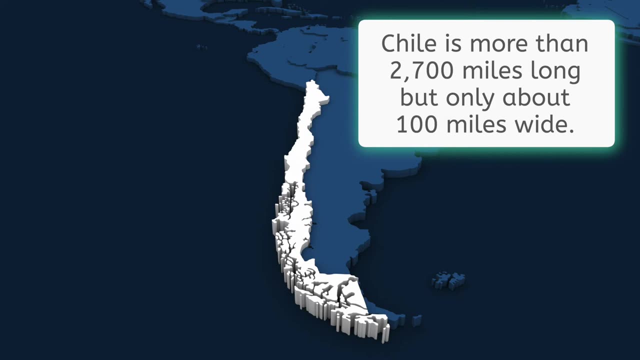 The nation of Chile is uniquely shaped as a long, narrow ribbon of land that is more than 2,700 miles long but only about 100 miles wide, as it runs from the northern part of the continent to the southern tip and south 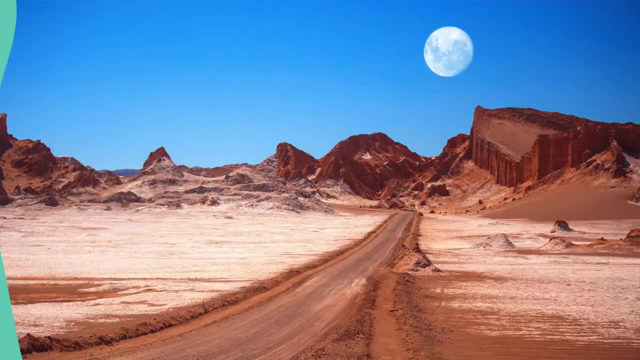 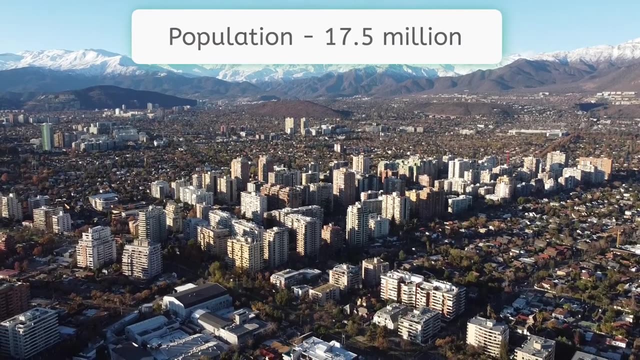 Chile is the only continent in Paragonia and the Tierra del Fuego. The Atacama Desert in the north is mostly uninhabited. As you'd expect, about three-fourths of Chile's estimated 17.5 million people reside in the central valley between the Andes and the Pacific coast. 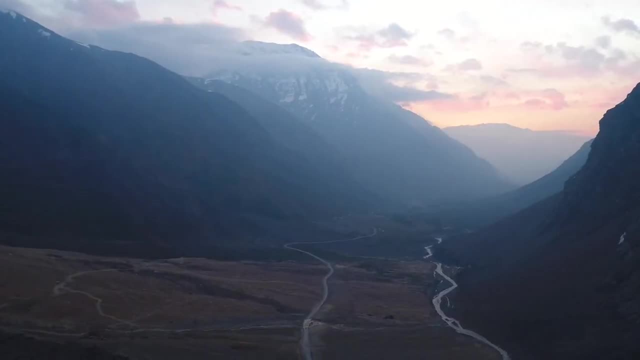 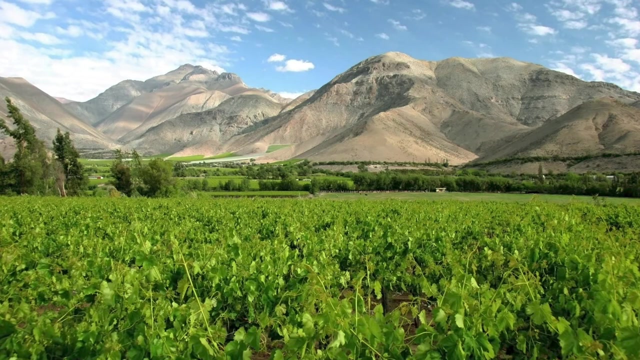 The area is blessed with fertile river basins that produce prodigious amounts of fruits and vegetables. Because of its location in the southern hemisphere, Chile's summer corresponds with winter in the US and Europe. The timing allows its summer crops to be available for the winter markets of their northern neighbors.